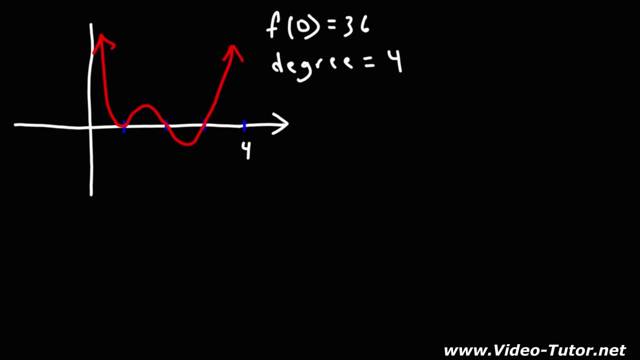 how can we find and write a polynomial function that corresponds to this graph? So we have an x-intercept at 1, another x-intercept at 2, and another one at 3.. So we can write the zeros of the polynomial function, which are x equals 1,, x equals 2, and x equals 3.. 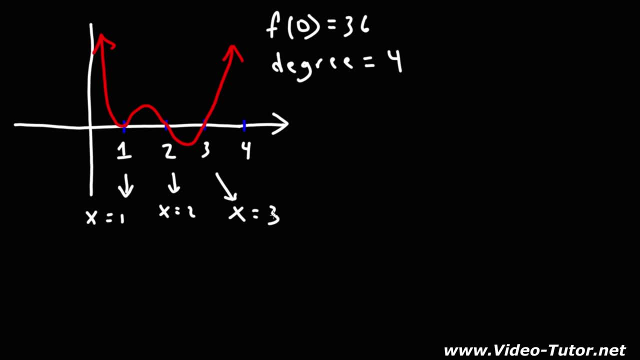 Now, once you know the zeros of the polynomial function, you can write the factors. So for this zero, x equals 1, the factor is going to be x minus 1.. If you set x minus 1 equal to 0 and solve for x, you'll get that x will have a value. 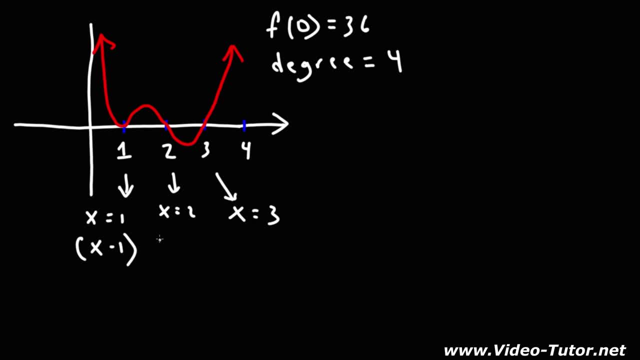 of positive 1.. When x is equal to positive 2, the factor that corresponds to that is going to be x minus 2.. And for x equals 3, the factor that corresponds to that one is x minus 3.. Now we need to pay attention to the multiplicity of each zero. 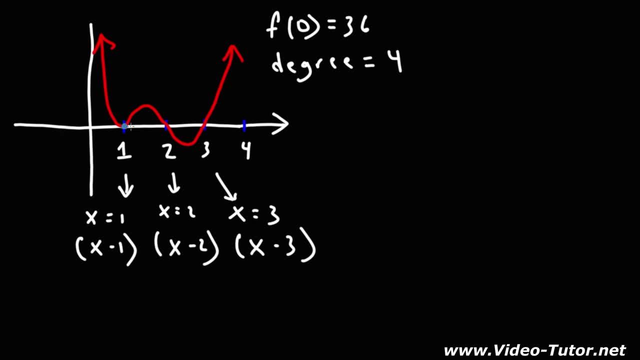 If we focus on the graph, notice that at this point, at x equals 1, the curve it touches the x-axis, But at x equals 2, it crosses over the x-axis. What we need to know is that when it crosses over, the multiplicity is odd. Typically, the multiplicity will be 1,. 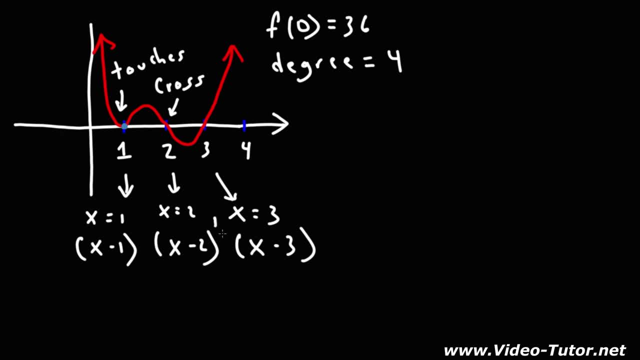 not 3. When it touches the x-axis but doesn't cross over, the multiplicity will be even most likely: 2. Here it crosses over, so the multiplicity is going to be 1.. Now how do you know if it's 1 or 3, or 2 or 4?? The answer has to do with the degree of the polynomial. 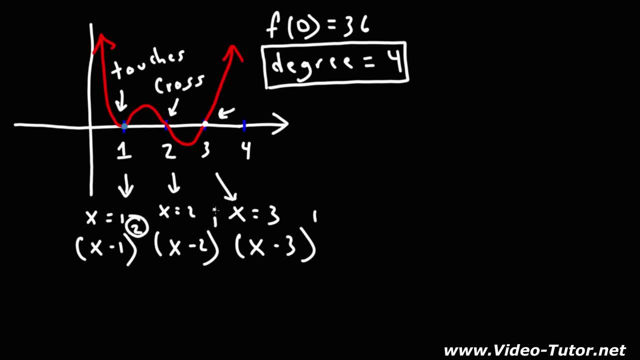 function These exponents. the sum of the multiplicity values must equal the overall degree of the polynomial. So 2 plus 1 plus 1 is 4.. We're good If we were to try the other possibilities. it won't work. For instance, for this one at x equals 1, it touches which? 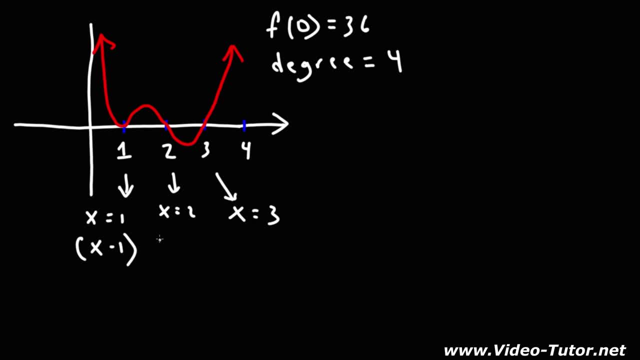 of positive 1.. When x is equal to positive 2, the factor that corresponds to that is going to be x minus 2.. And for x equals 3, the factor that corresponds to that one is x minus 3.. Now we need to pay attention to the multiplicity of each zero. 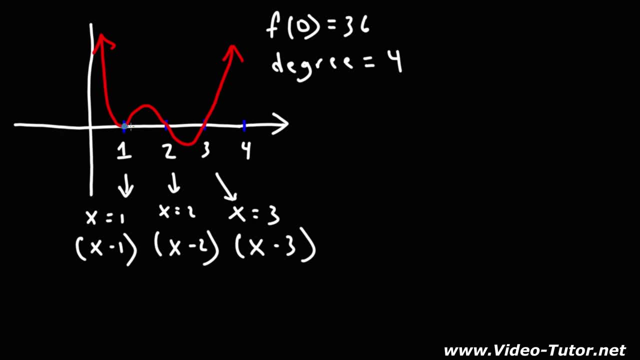 If we focus on the graph, notice that at this point, at x equals 1, the curve it touches the x-axis, But at x equals 2, it crosses over the x-axis. What you need to know is that when it crosses over, the multiplicity is odd. Typically, 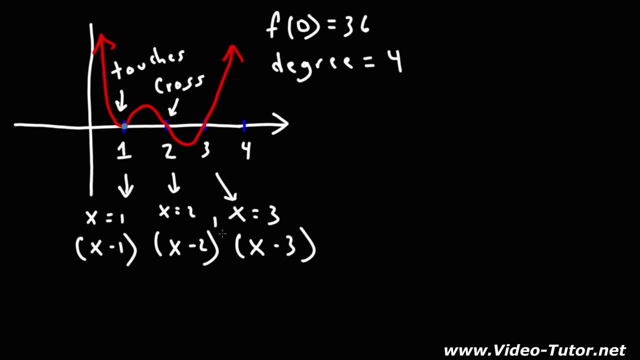 the multiplicity will be 1.. If not, it will be 0.. When x equals 1,, the multiplicity will be 0.. 3. When it touches the x-axis but doesn't cross over, the multiplicity will be even. 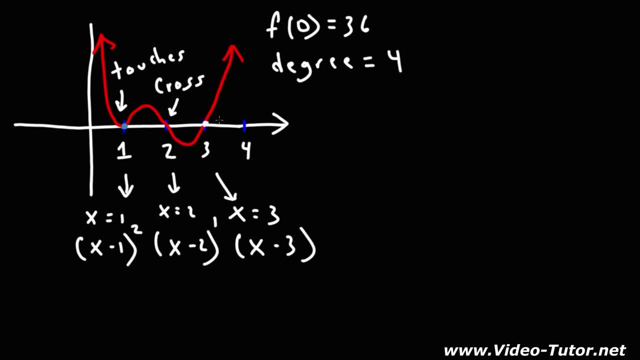 most likely 2.. Here it crosses over, so the multiplicity is going to be 1.. Now how do you know if it's 1 or 3, or 2 or 4? The answer has to do with the degree of the. 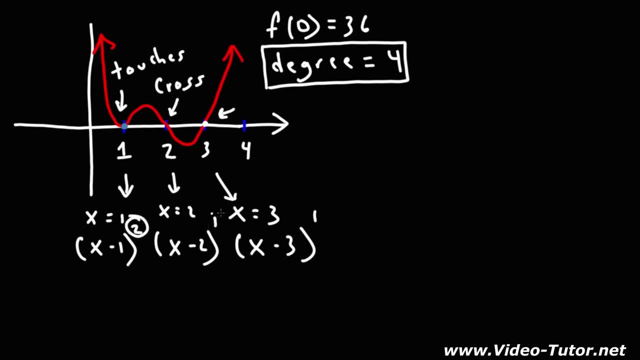 polynomial function. These exponents, the sum of the multiplicity values, must equal the overall degree of the polynomial. So 2 plus 1 plus 1 is 4, we're good. If we were to try the other possibilities, it won't work. For instance, for this one at: x equals 1, it touches 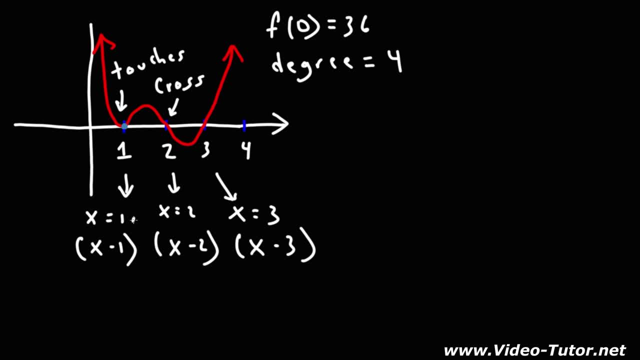 which means it's going to be a 2 or 4.. If we try a 4, that's already going to be too much, So this has to be a 2,, which means these: they have to be a 1 in order for. 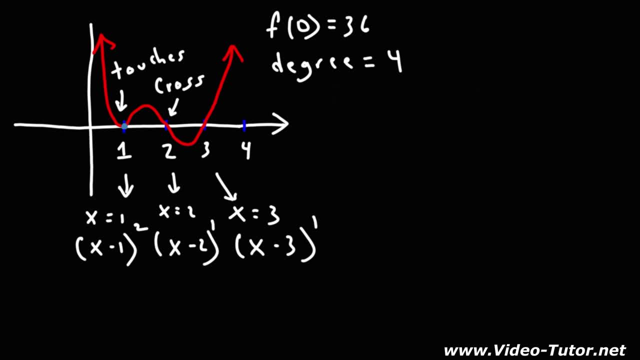 to be a fourth degree polynomial. So now, at this point, what we need to do is set this equal to y and we need to add a coefficient in front of the polynomial function, Using the y intercept. using this point 0, comma 36,, we need to solve for the constant a. So what we're going? 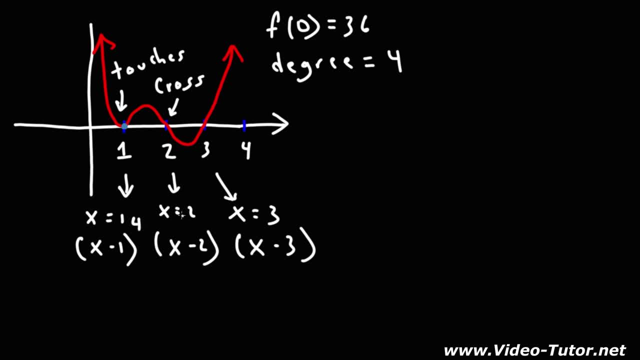 means it's going to be a 2 or 4.. If we try a 4, that's already going to be too much. So this has to be a 2,, which means these: they have to be a 1 in order for it to be. 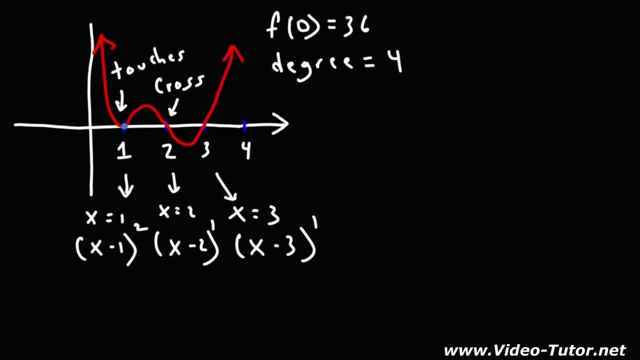 a fourth degree polynomial. So now, at this point, what we need to do is set this equal to y and we need to add a coefficient in front of the polynomial function, Using the y-intercept, using this point, 0 comma 36.. 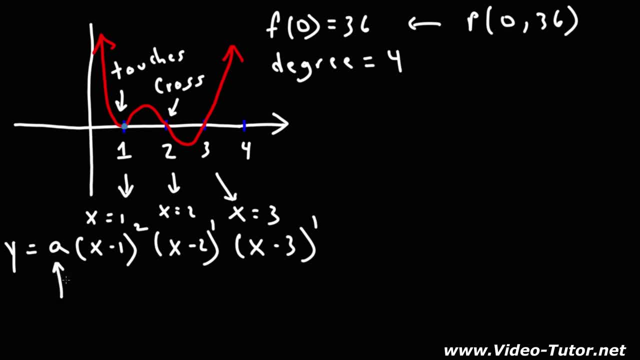 We need to solve for the constant a. So what we're going to do is we're going to replace x with 0, and we're going to replace y with 36.. So we're going to have: 36 is equal to. 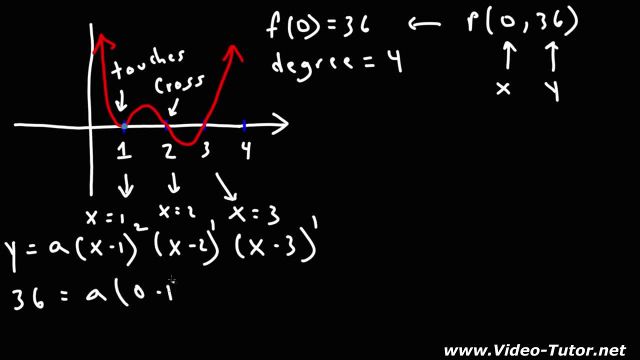 a times 0 minus 1, squared times 0 minus 2 times 0 minus 3.. Negative 1 is equal to a times 0 minus 2 times 0 minus 3.. Negative 1 squared is just 1.. 0 minus 2 is negative 2.. 0 minus 3 is negative 3.. 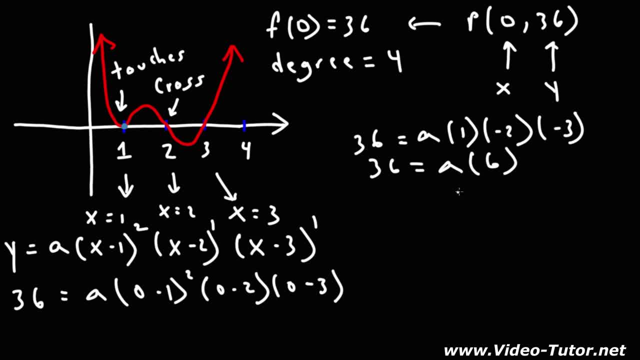 Negative 2 times negative, 3 is 6.. And 36 divided by 6 is 6.. So a is equal to 6.. Now that we have our a value, we can go ahead and write the equation of the polynomial function. 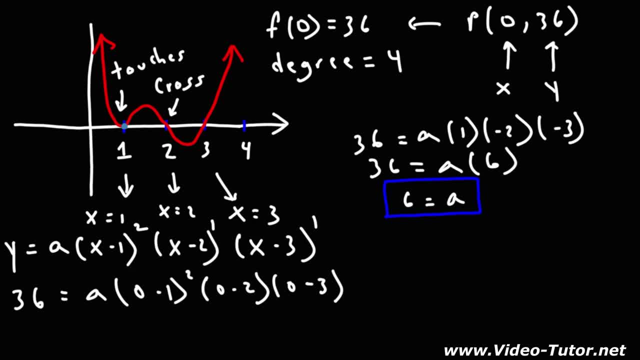 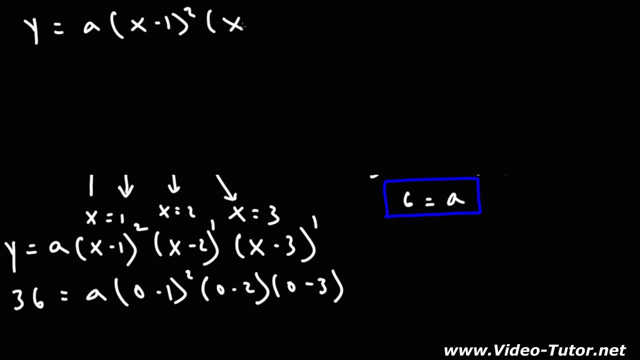 in factored form. So it's going to be: y is equal to a times x minus 1 squared. I mean we can replace a with 6. I forgot to do that. So it's 6 times x minus 1 squared. times x minus 2. times x minus 3.. 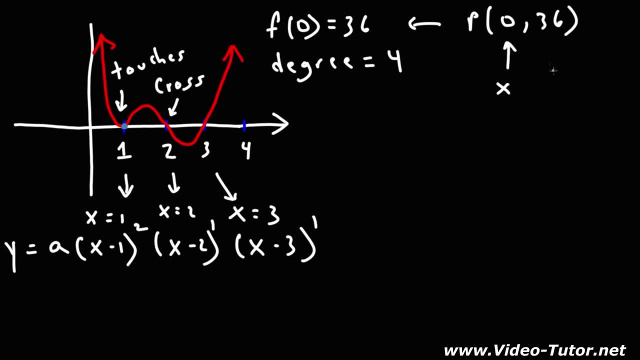 to do is we're going to replace x with 0, and we're going to replace y with 36.. So we're going to have: 36 is equal to a times 0 minus 1, squared times 0 minus 2, times 0 minus 3.. 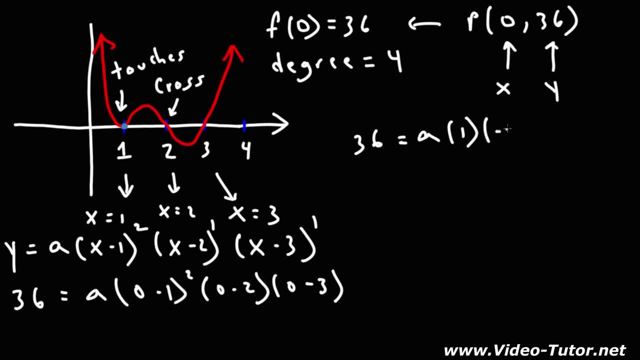 Negative 1 squared is just 1.. 0 minus 2 is negative, 2.. 0 minus 3 is negative, 3.. Negative 2 times negative: 3 is 6. And 36 divided by 6 is 6.. So a is equal to 6.. 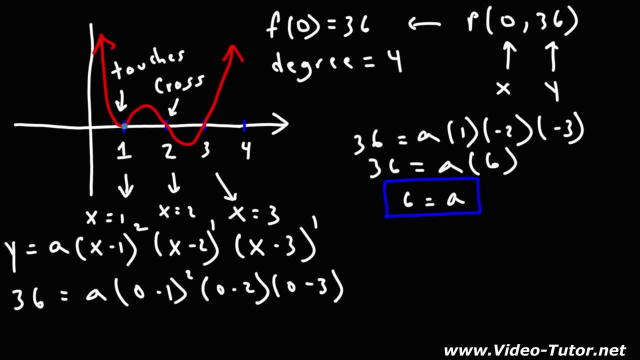 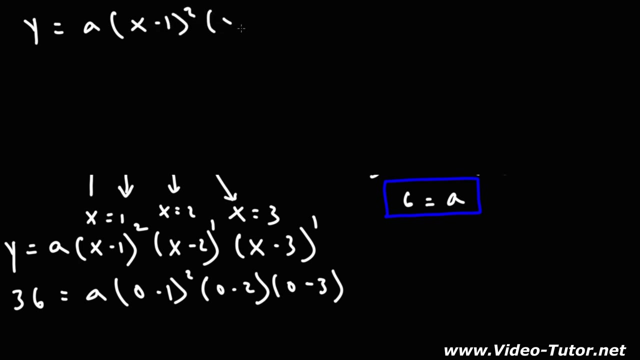 Now that we have our a value, we can go ahead and write the equation of the polynomial function in factored form. So it's going to be: y is equal to a times x minus 1 squared. I mean we can replace a with 6.. 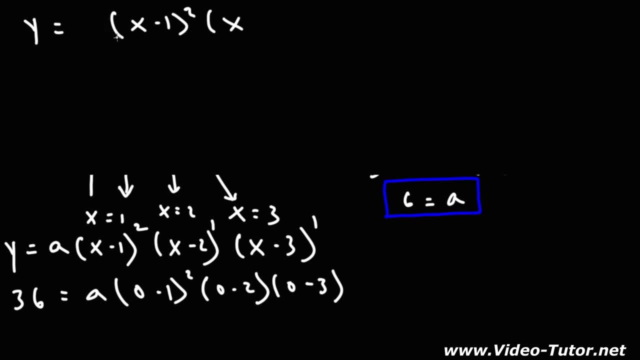 I forgot to do that. So it's 6 times x minus 1, squared times x minus 2 times x minus 3.. So this is the answer in factored form. Now sometimes you may need to convert the answer from its factored form to standard. 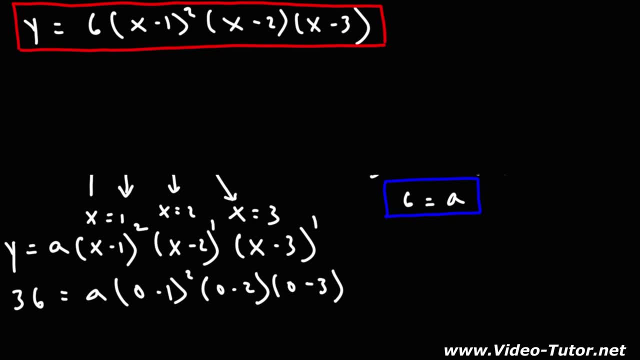 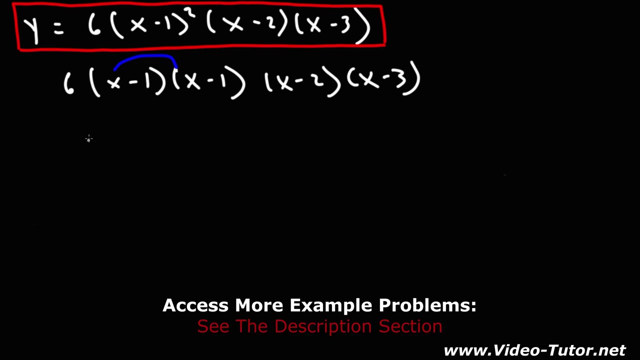 form. To do that, we just need to FOIL So x minus 1 squared. I'm going to expand that. So let's begin by FOILing these two factors. So this is going to be x times x, which is x squared. 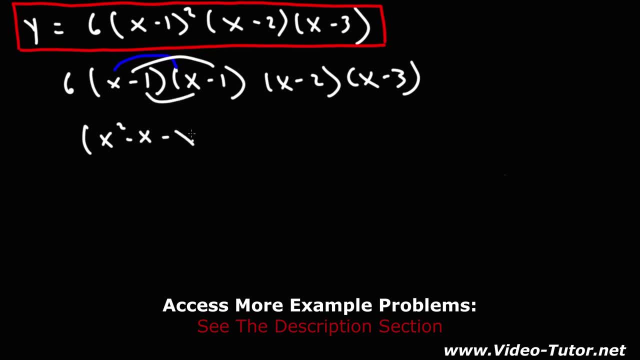 And then this is going to be negative: x negative, x negative, 1 times negative: 1. That's positive, 1. Now let's FOIL the remaining two factors, So we're going to have x squared. This is going to be negative 3x. 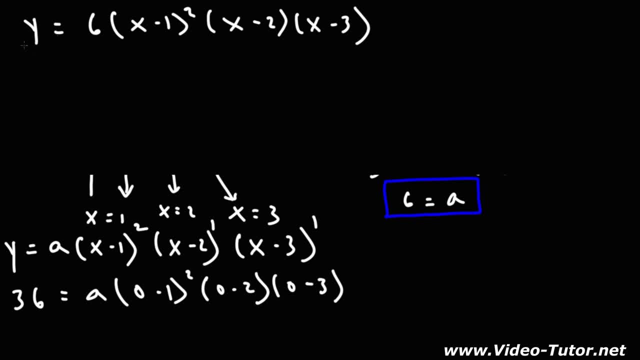 So this is the answer in factored form. Now sometimes you may need to convert the answer from its factored form to standard form. To do that we just need to FOIL: So x minus 1 squared. I'm going to expand that. 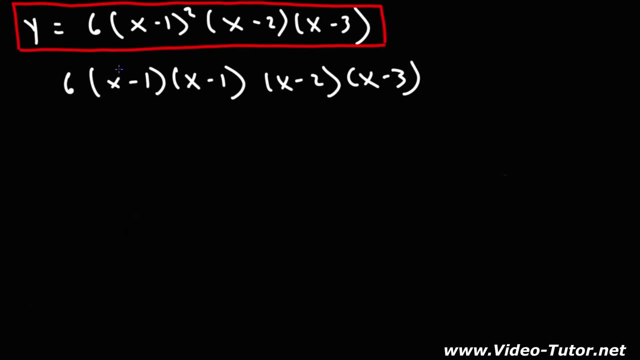 So let's begin by FOILing these two factors. So this is going to be x times x, which is x squared, And then this is going to be negative, x, negative, x, negative, 1 times negative, 1, that's positive. 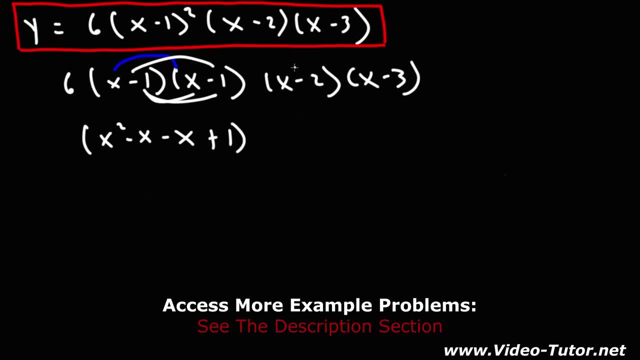 1. Now let's factor the remaining two. So let's do that, I mean let's FOIL the remaining two factors. So we're going to have x squared. this is going to be negative 3x and then negative 2x. negative 2 times negative, 3 is positive 6.. 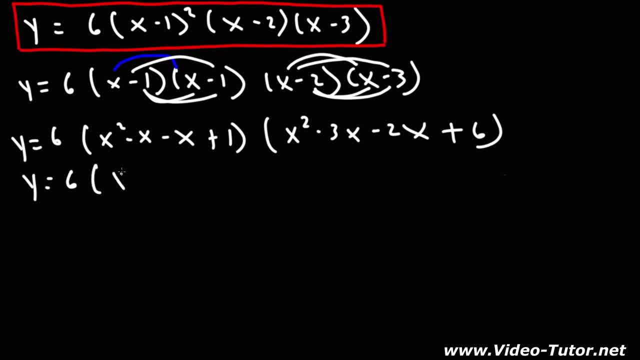 Now let's go ahead and simplify. Negative x minus x is negative 2x, And negative 3x minus 2x that's going to be negative 5x. So we have this All right. this one is going to be a little bit longer. 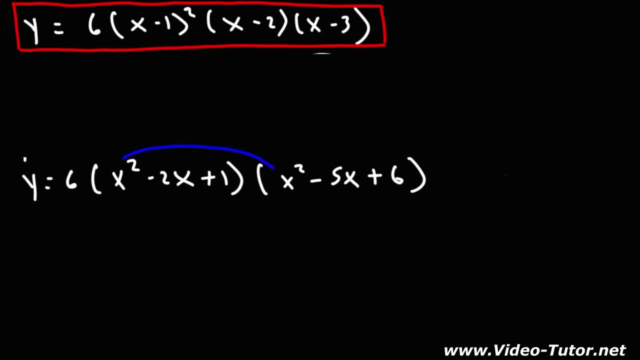 So now let's go ahead and FOIL what we have now: X squared times x squared, that's going to be x to the fourth, And then x squared times negative 5x, that's going to be negative 5x. And then x squared times negative 5x, that's going to be negative 5x. 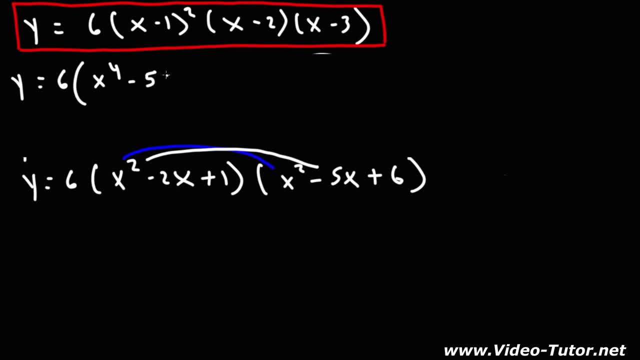 So we have this Negative 5x cubed And then x squared times 6, that's going to be 6x squared. Now I'm going to line it up in an interesting way so that it'll be easy to combine like: 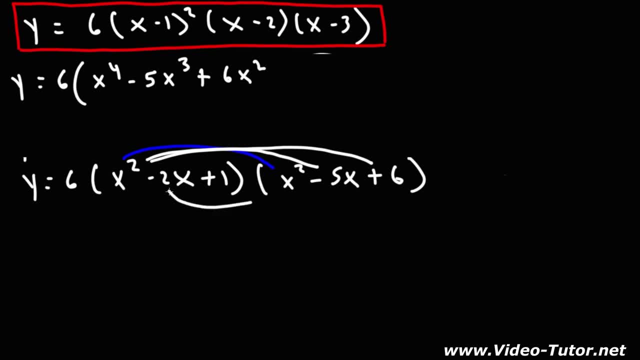 terms. Now let's move on to negative 2x. Negative 2x times x squared: that's negative 2x squared, and I'm going to put that here. Negative 2x times x squared: that's negative 2x squared, and I'm going to put that here. 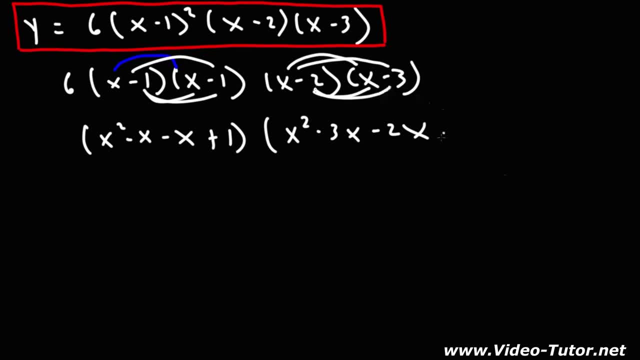 And then negative 3x, Negative 2x, Negative 2 times negative, 3 is positive 6.. Now let's go ahead and simplify: Negative x minus x is negative 2x, And negative 3x minus 2x, that's going to be negative 5x. 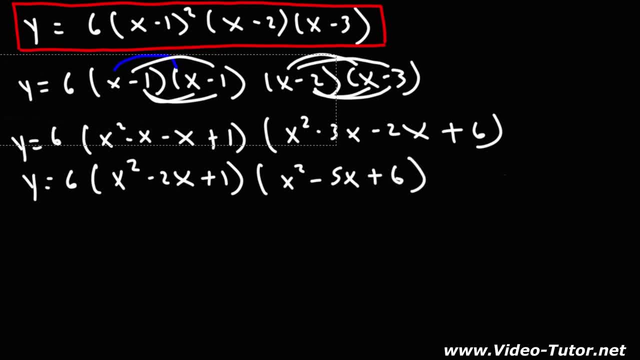 So we have this. We have this. All right, this one is going to be a little bit longer, So now let's go ahead and FOIL what we have now: x squared times, x squared, That's going to be x to the fourth. 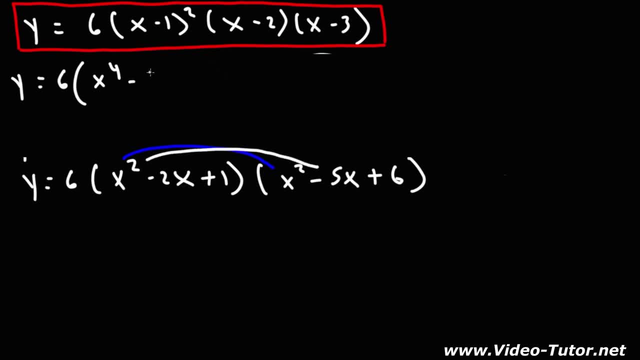 And then x squared times negative 5x. That's going to be negative 5x cubed. And then x squared, And then x squared, x squared times x squared. x squared times 6,, that's going to be 6x squared. 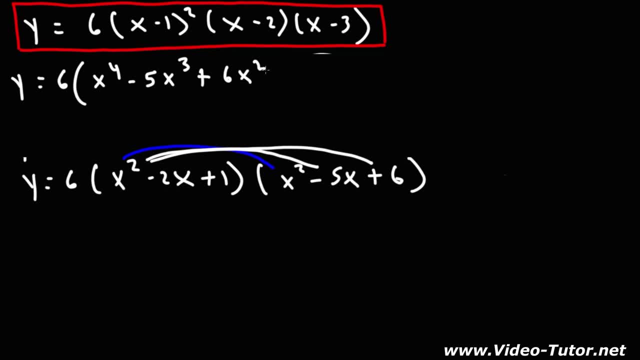 Now I'm going to line it up in an interesting way so that it'll be easy to combine like terms. Now let's move on to negative 2x Negative 2x times x squared. that's negative 2x squared, and I'm going to put that here. 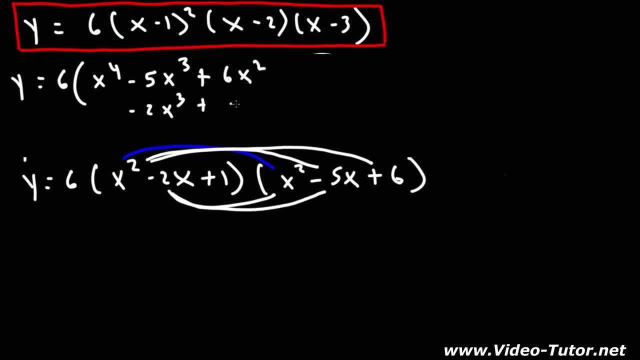 Negative 2x times negative 5x, it's positive 10x squared. And then negative 2x plus 6, that's negative 12x. And then here we have 1 times x squared. so that's positive x squared or just 1x squared. 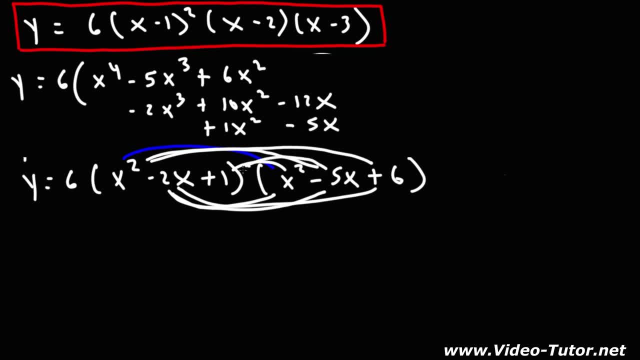 And then 1 times negative 5x, which will be negative 5x, and the 1 times 6 is 6.. So we can bring this down: Negative 5 plus negative 2, we're adding, by the way, 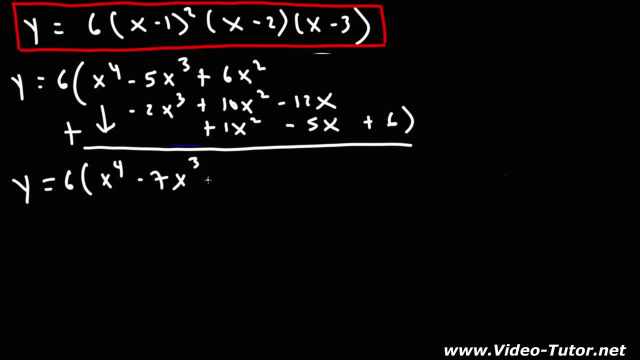 it's going to be negative: 7.. 6 plus 10 plus 1, that's 17.. Negative. 12 minus 5, that's also 17,, but negatives. Now, the last thing we need to do is we need to distribute this. 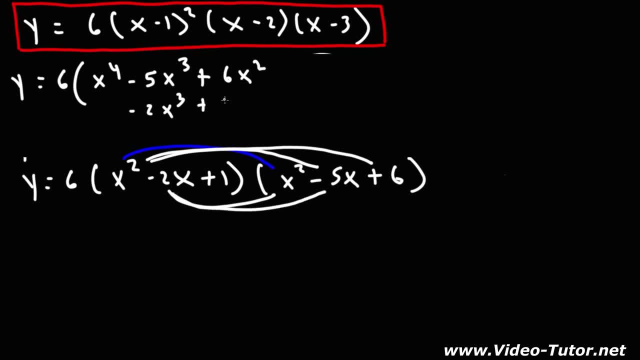 Negative 2x times negative 5x, that's positive 10x squared. And then negative 2x plus 6, that's negative 12x. And then here we have 1 times x squared. so that's positive x squared or just 1x squared. 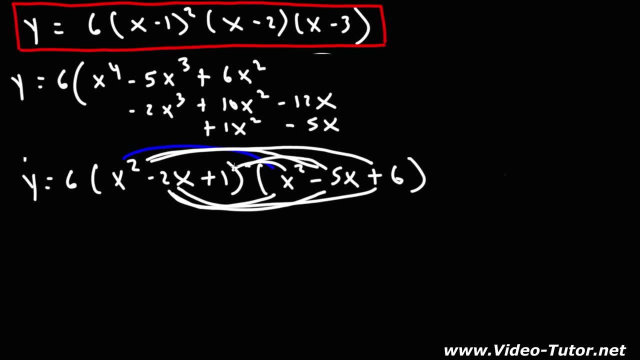 And then 1 times negative 5x, which will be negative 5x, And the 1 times 6 is 6.. So we can bring this down: Negative 5 plus negative 2. We're adding, by the way, 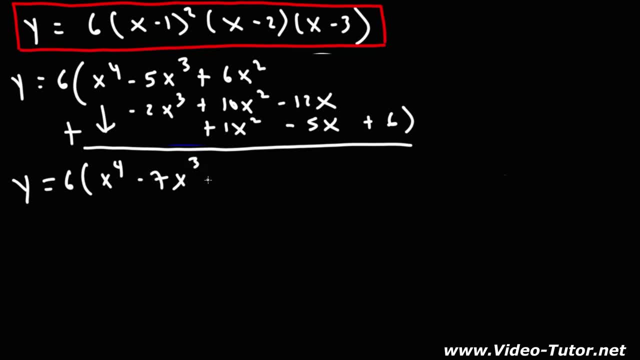 It's going to be negative: 7.. 6 plus 10 plus 1, that's 17.. Negative. 12 minus 5, that's also 17,, but negatives. Now, the last thing we need to do is we need to distribute the 6.. 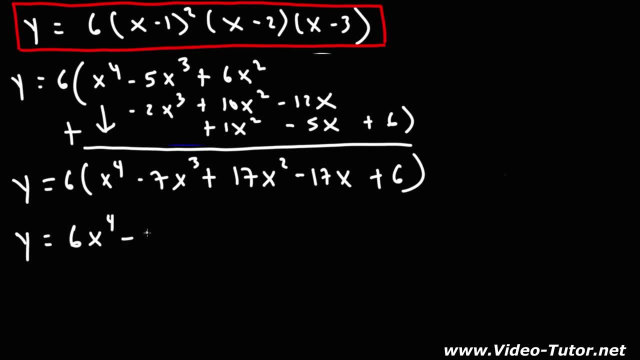 So it's going to be 6x to the 4th, 6 times negative 7, that's going to be negative 42. And then times x cubed Now 6 times 17.. 6 times 10 is 60.. 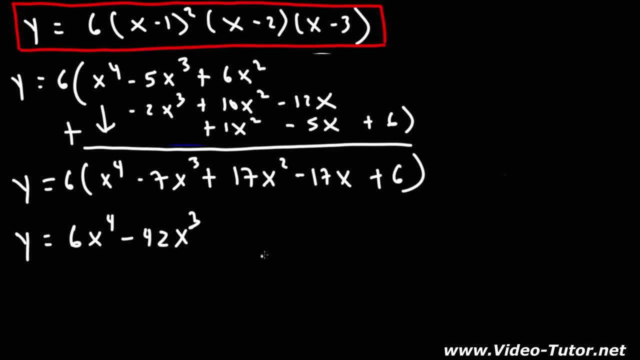 6 times 7 is 42.. 60 plus 42 is going to be, So this is going to be positive 102x squared And then negative 102x. Finally, 6 times 6 is 36.. So, if I didn't miss anything, 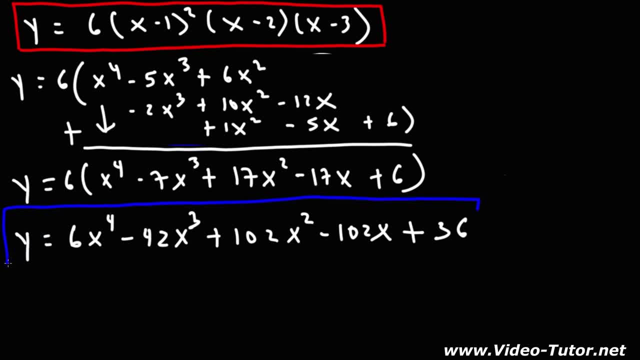 if I didn't miss any negative signs or didn't mess up any multiplication. this is what the answer should be in standard form. So if you have a test, you need to pay attention to the directions on the test, because sometimes you don't know. 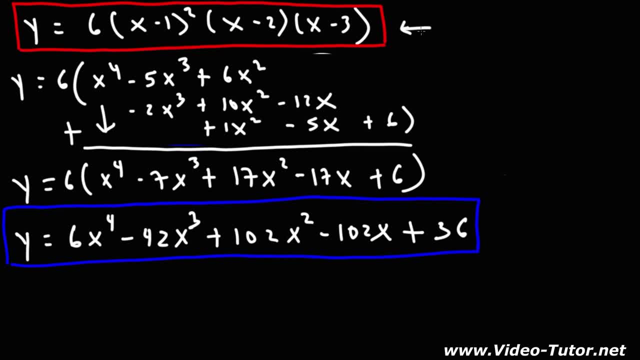 and sometimes your teacher or professor. they may want you to write the answer in factored form. If that's the case, the problem is going to be quick and simple. You could finish it quickly. If not, you may have to put it in standard form. 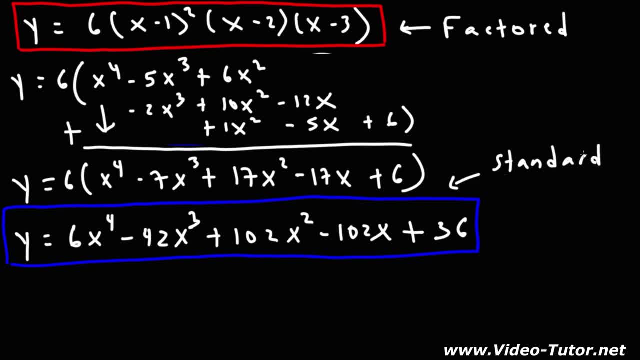 which that's going to take some time. So that's basically it for this video. By the way, for those of you who want more content relating to polynomial functions, like how to graph them and things like that, or how to factor them,